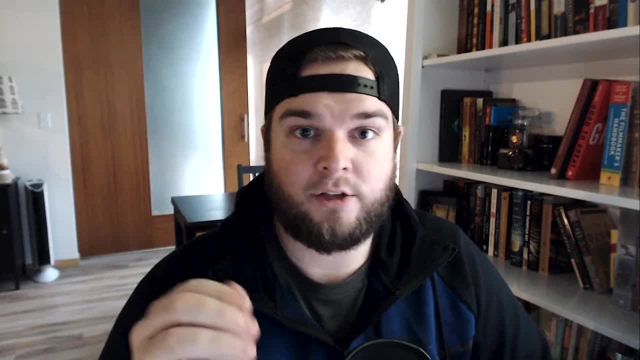 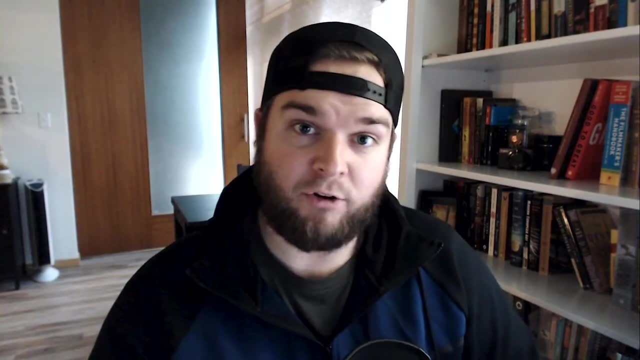 and have more engaging content though customized video to those audiences. So if you look up insights that you can see through the data that those people care about, that will help you determine your content and get you down the road to those more, better and more relevant videos. 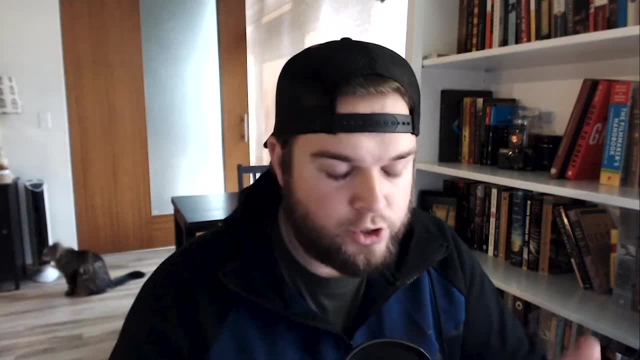 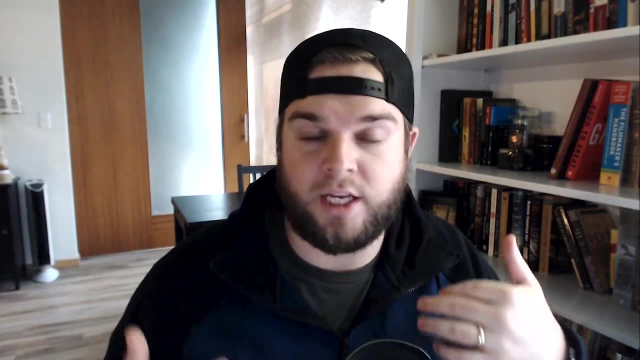 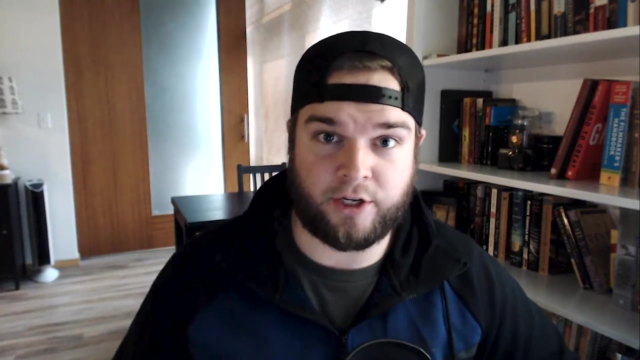 There's my wife's cat. So there's no better example than my professional world that I live in, which is with advertisers, as to how they use and utilize this information. Now, the benefit that advertisers have over small businesses, entrepreneurs or creators like yourself. 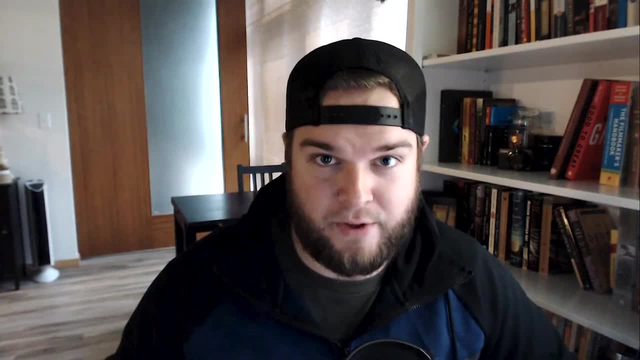 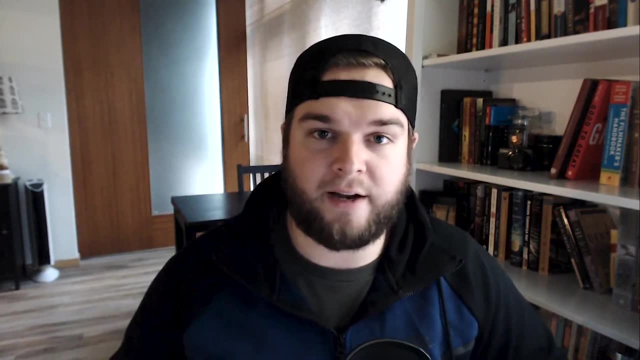 is that they pay, in some cases, millions and millions of dollars to have access to syndicated research platforms where there is a really stable, awesome amount of data that provides countless- I can't even tell you how much information where people are signing up. 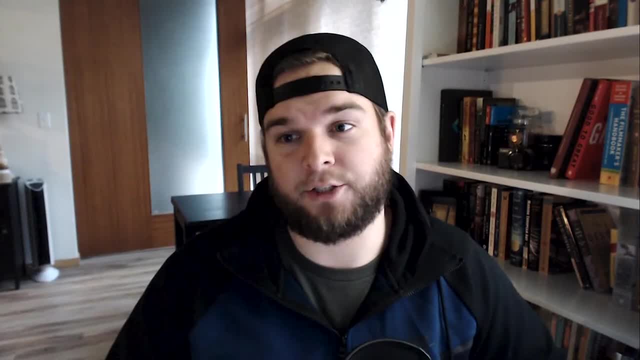 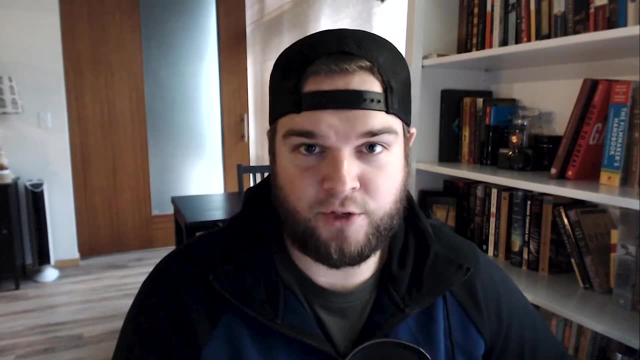 to be part of a panel or research studies where we can get this information. But, like I said, the problem is that these aren't accessible to you and me. But there are some free tools out there that allow us to get almost all the way there right. So again, it doesn't matter if 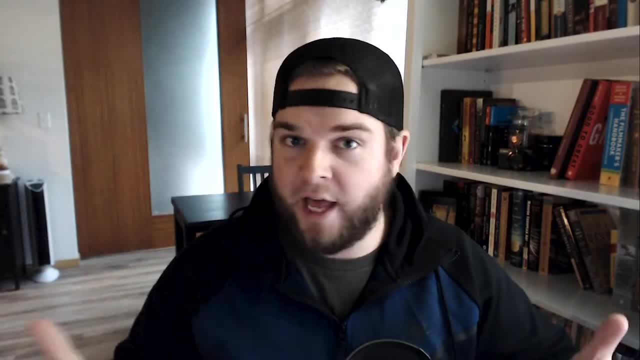 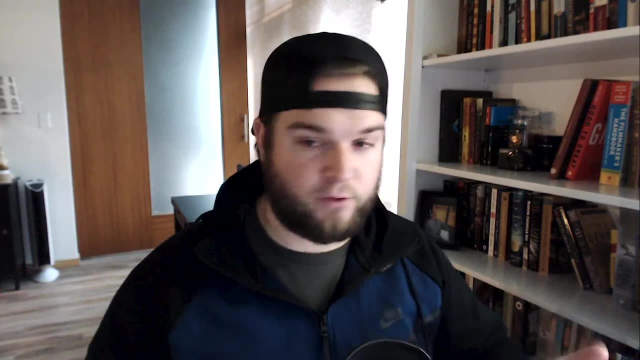 you're on Instagram or Twitter or Facebook or YouTube or what have you- this platform that I'm about to go through in these insights are super, super helpful. So if you're on Instagram or Twitter, this is super relevant. So the first thing I'm going to do is just click over to this. 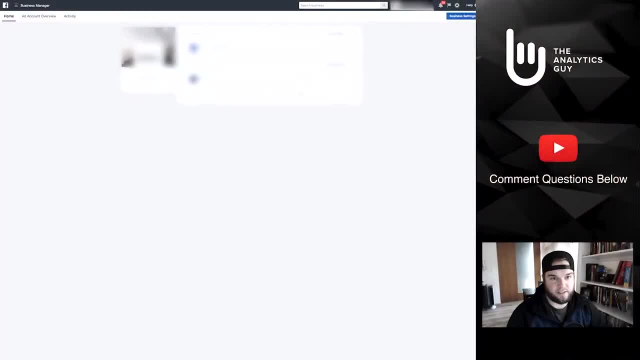 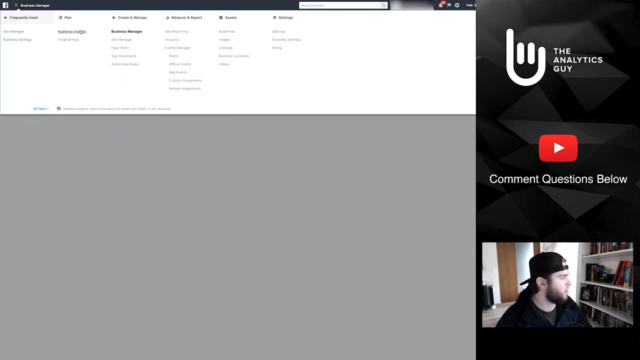 tool and it is actually Facebook Audience Insights. So if you go to businessfacebookcom, so you'll see that in the description below you will come to a page like this: If you come to the little buttons up here, go to More Tools and then the Audience Insights, you come to a page. 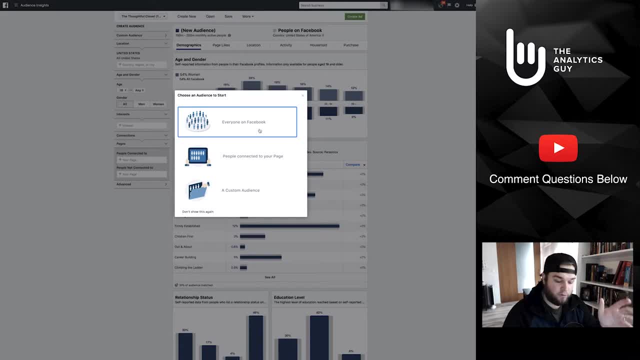 that looks just like this. Now, it gives you some information here. So some of us have Facebook pages, or maybe that's what you do. as you focus on Facebook, You can actually see what are the people that are just connected to my page. if you want to build a custom audience, or if you, 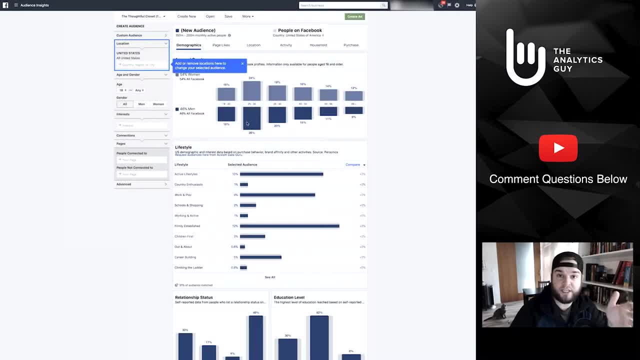 just want everyone on Facebook. Now I'm going to click everyone on Facebook and the reason why. okay, some of the largest syndicated research platforms in the world- ie, Nielsen, Miller, Brown- they back up their data and information from Facebook data. So whether some of you know, 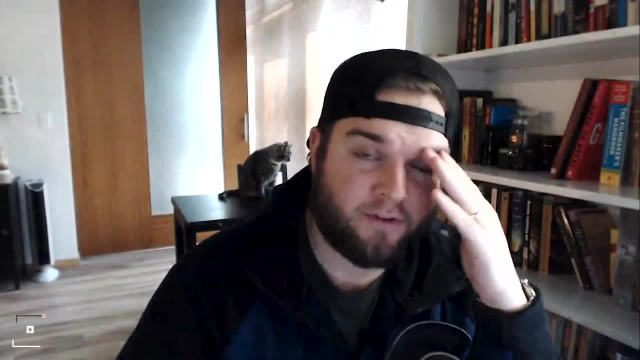 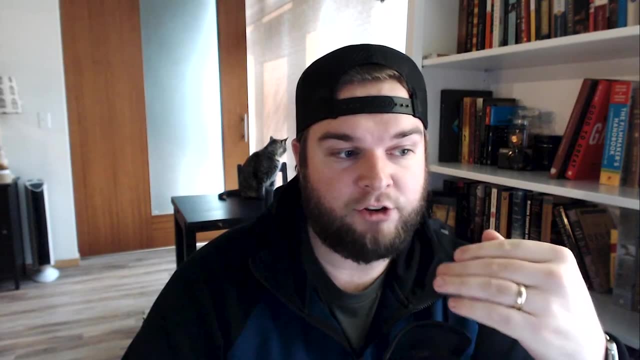 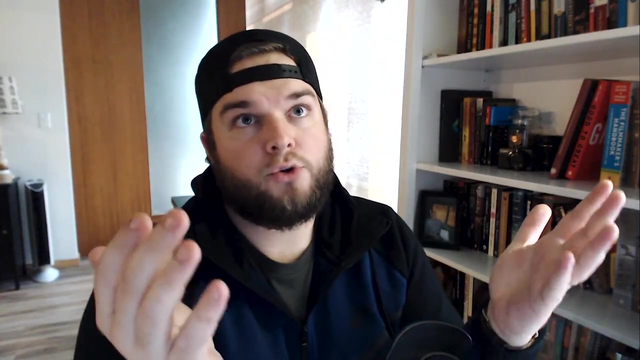 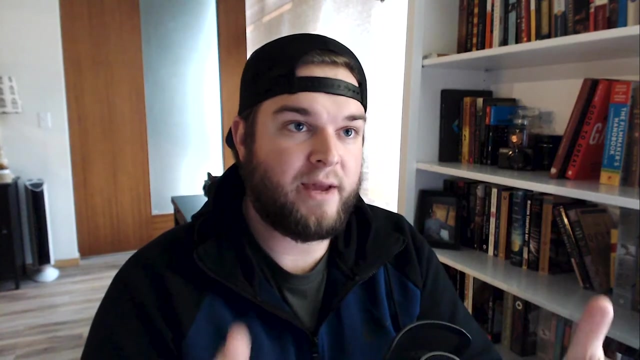 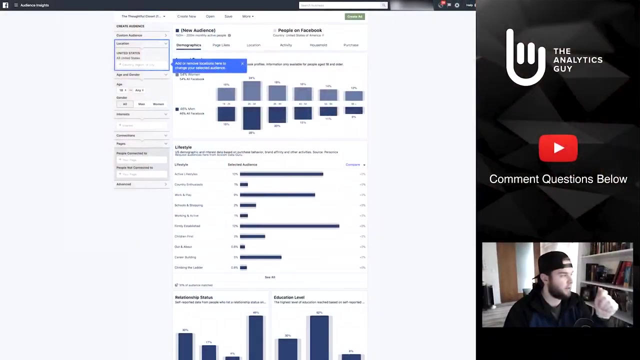 this or not Facebook does. They do not sell personal, identifiable information, but they will say: you know things like: do you own a pet, like is on the table behind me, or what are these different types of behaviors that they may see with you on Facebook, and can they create buckets for those? And that's what this platform is. So let's dive back in there. 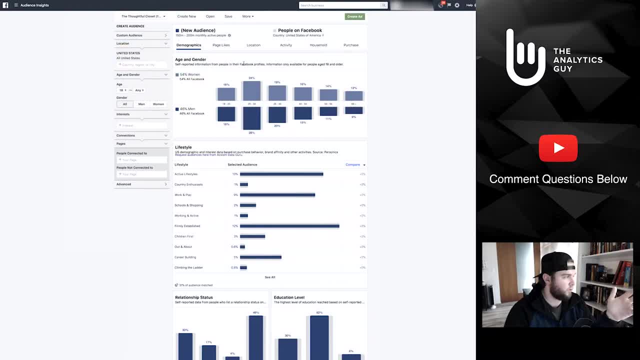 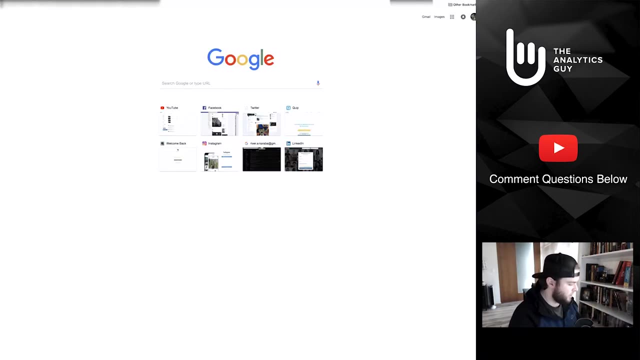 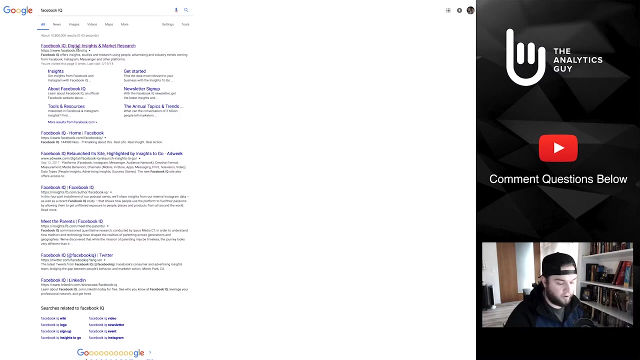 So you'll see right here that this is just kind of released for everyone. So they have the demographic information page, likes, location activity, all kinds of purchase activity, all kinds of really good stuff in here. The second tool that I'm actually going to go through is a tool called Facebook IQ. So Facebook IQ, So I'm going to call Facebook IQ. I'm just going to show you how easy it is to get to that. You just Google search, You can click on it right here, And Facebook IQ is a ton of research that Facebook has actually done across advertisers. 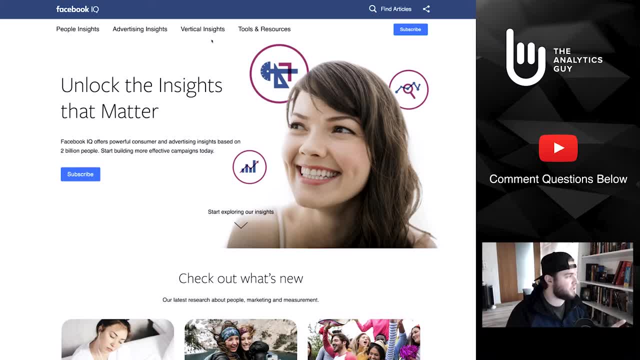 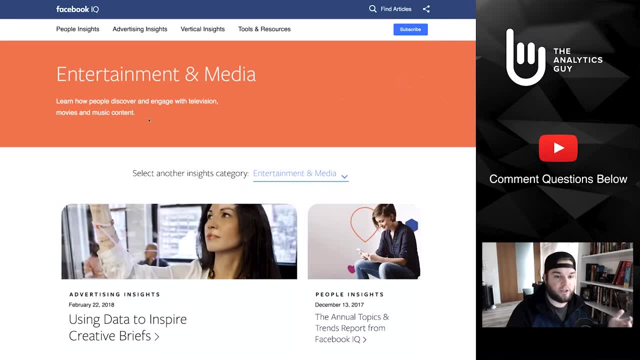 right across their platform And there's all kinds of really good insights. So if you go up here and you have a vertical that you are particularly interested in- So maybe it's entertainment and media Right- You can click in here and they'll have all kinds of different studies or information that you could have in here. 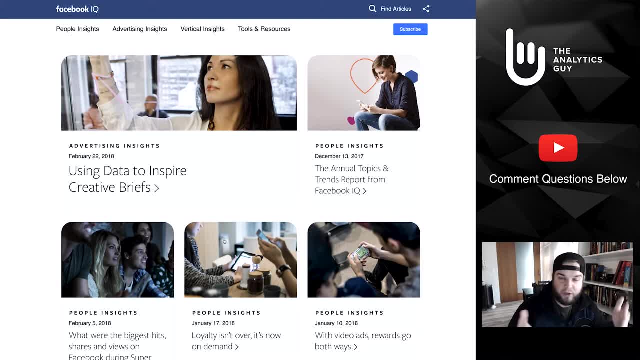 One of my favorite things for you guys is just using the information that I have from the advertising world and providing it to you because you don't know it exist. This is a big one, But let's go back to that audience insights tool and talk about how exactly would we use this. But let's go back to that audience insights tool and talk about how exactly would we use this. But let's go back to that audience insights tool and talk about how exactly можно usows dollars if we really want that news to get to one of these members who are more excited than probably 150 are in the audience. 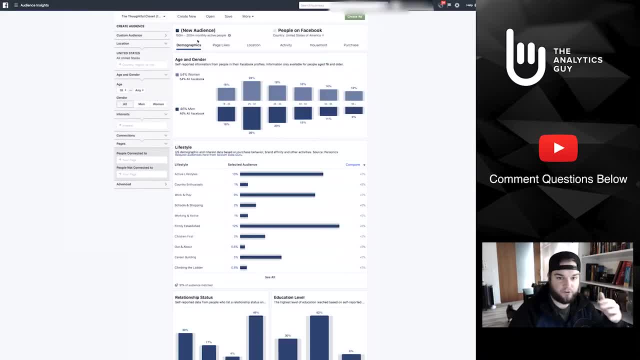 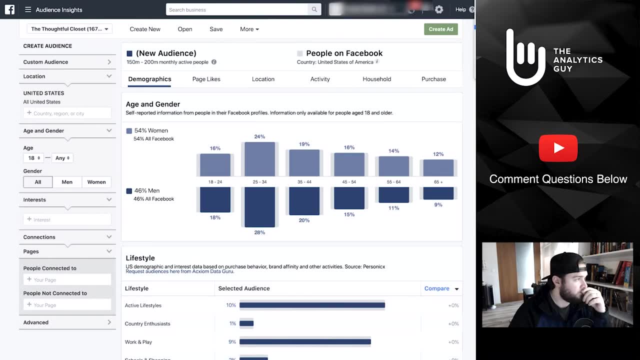 Insights tool and talk about how exactly would we use this. The first thing I'm going to do is go ahead and zoom in here a little bit, just so you can see that. Hopefully you guys can see that a little better now. The biggest thing here that you can really start to zero in on is emulating the data. 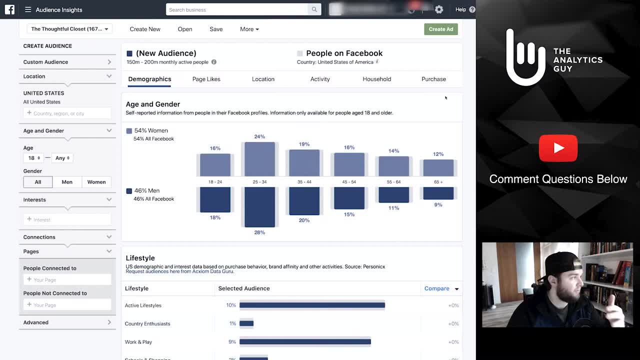 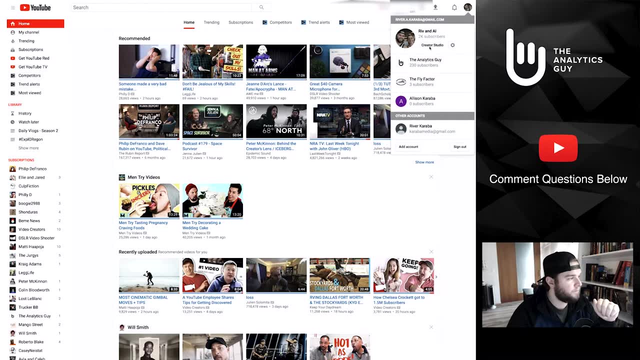 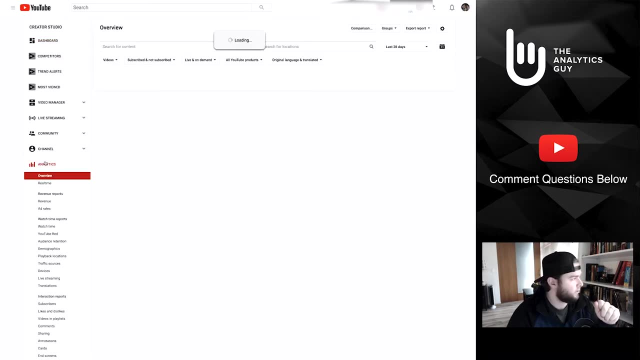 that you're seeing Again. go into those native platforms First. let's go into YouTube, for example. We're going to go into YouTube, We're going to navigate up to our Creator Studio, We're going to come up here, come into Analytics and we're going to go into Demographics. 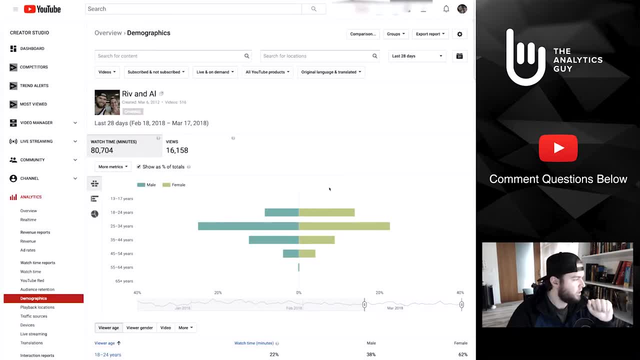 Demographics is going to default to a view that looks something like this: The view that you're looking at right now are males and females across this vlogging channel and the ages that you have here. You can dive into a ton of different information here, but just in looking at this right now, 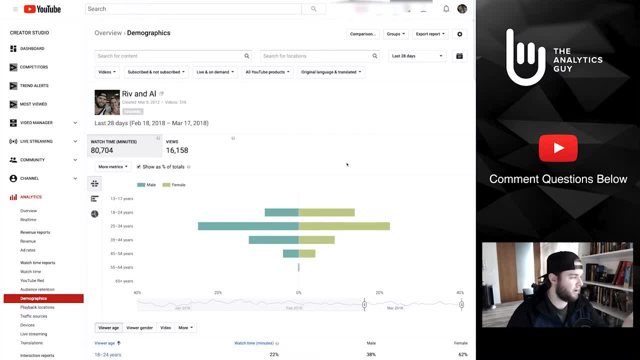 you can see that this audience is predominantly male, Probably 25 to 34, both male and female. Something that's kind of interesting here is that it skews: younger for female but older a little bit for male. but maybe we care about that bread and butter the most, that 25 to 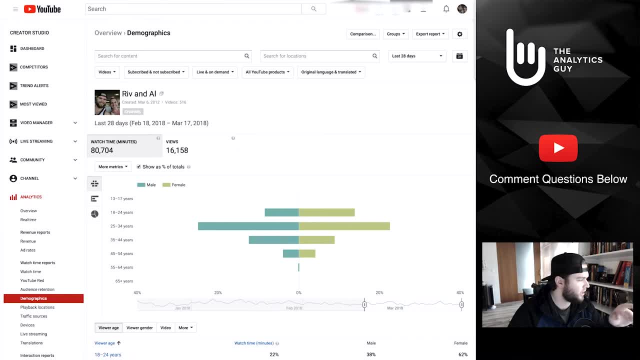 34. Now if anyone is watching who is part of my vlogging channel, you are all equally cared about, but for demonstration purposes we're going to pick that 25 to 34.. We can come back to the Audience Insights tool here on Facebook and remember this. 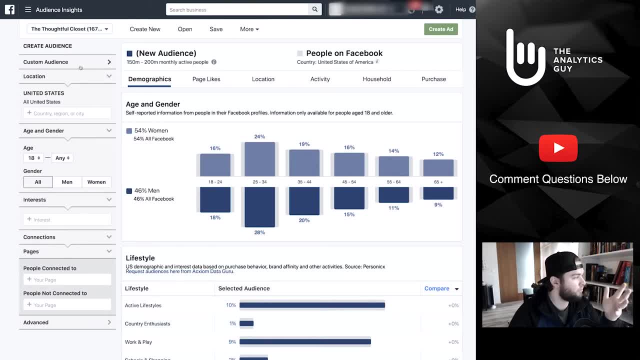 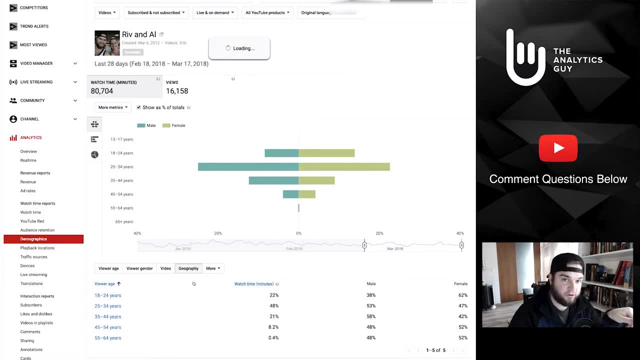 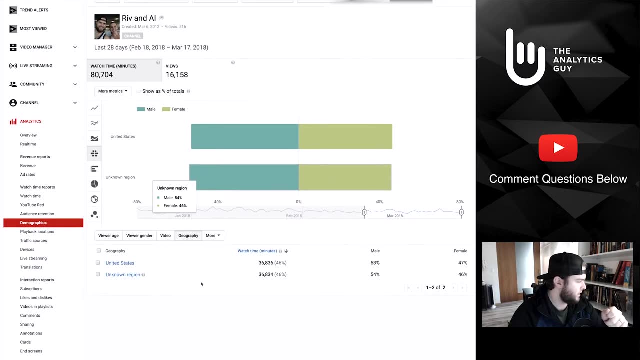 is everyone All right? Let's start to plug in some of this information. If we come back here, maybe we are wondering- you can click this down by geography. This is in the last 28 days. It looks like there is a pretty significant amount in the US and maybe for a video. 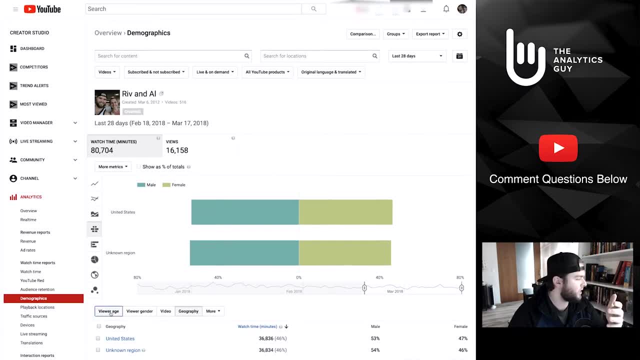 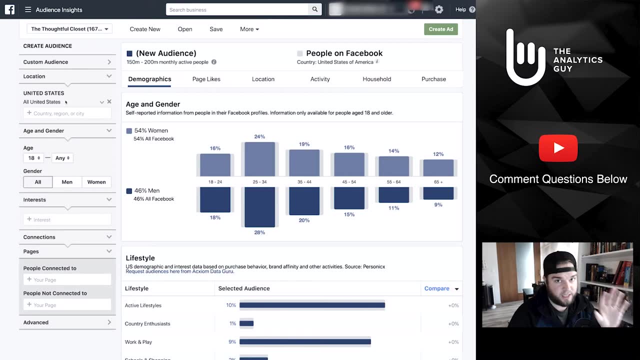 idea that I have. I want to look at just the US information. I may come up here and make sure that US is up here, or if you want to dig into a specific country, make sure you do that, because the insights are going to be different for each. 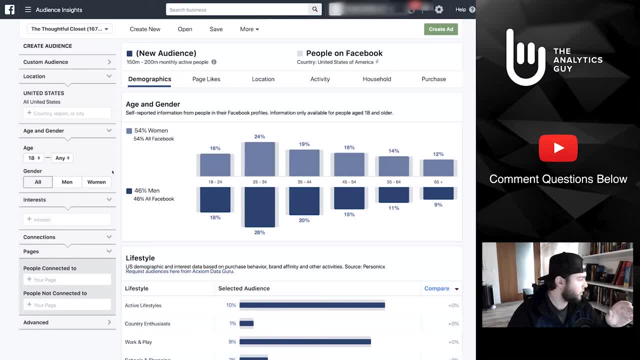 All right, That's a good thing for each country that you go into. Here we go. We can start to build this now. Let's say we want to do all genders and we're going to pick 25, go find it 34.. 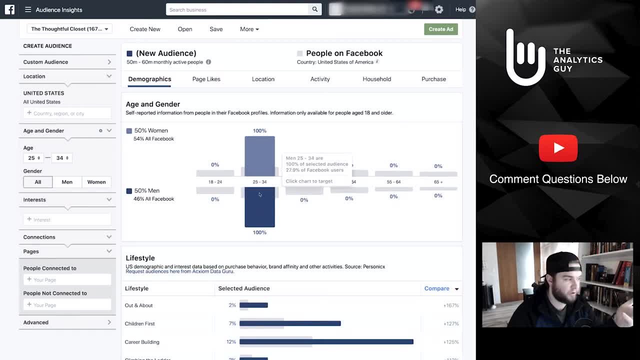 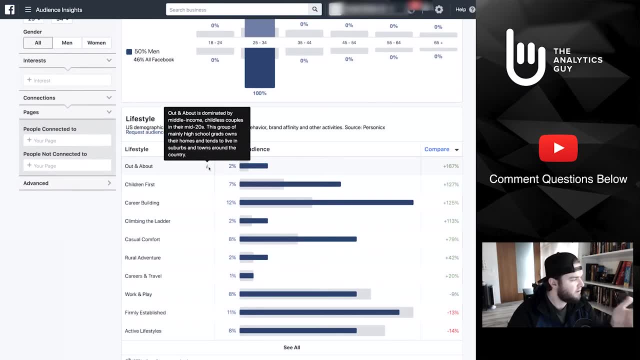 Okay, You can see already the information has changed, Obviously demographically. we're just talking about that single vertical, but down here there's all kinds of different information that you can start to get info about Out, and about what does that mean? 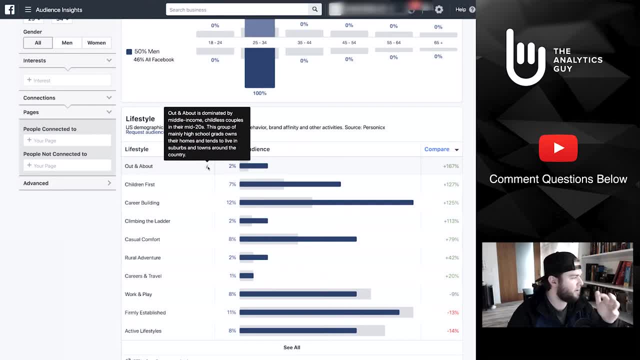 If you hover over here, it says Out and about is dominated by middle-income childless couples in their mid-20s. This group, mainly high school grads, owns their homes and tends to live in suburbs and towns around the country. Just random information here. 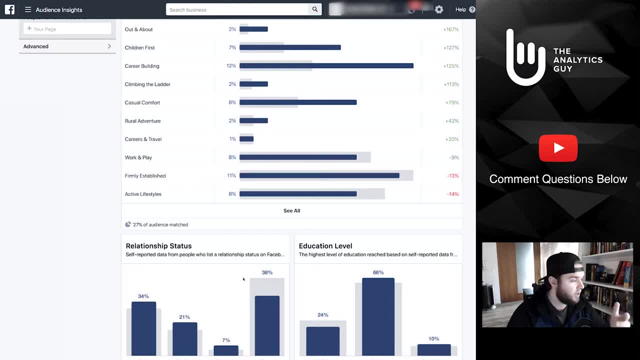 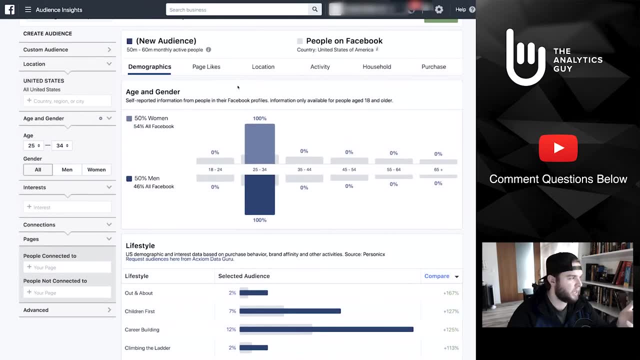 Relationship status, depending on how you're going to talk to these people, whether they're single, their education levels, job titles- all of this information you can see, depending on how you want to use. it is really interesting Page likes. 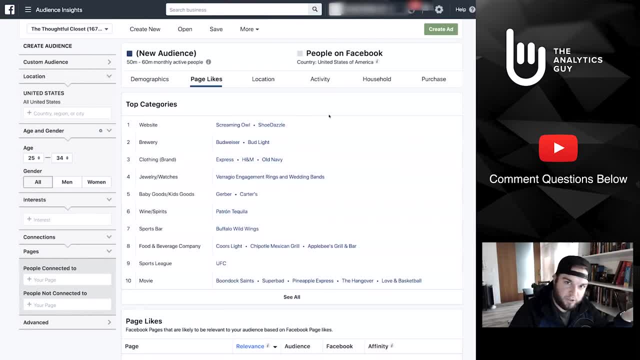 Here on Facebook. Again, these are the pages that they're liking on Facebook, but remember there is active tracking involved and so different pages that they interact with and things like that. Facebook is going to have that syndicated research free for you. 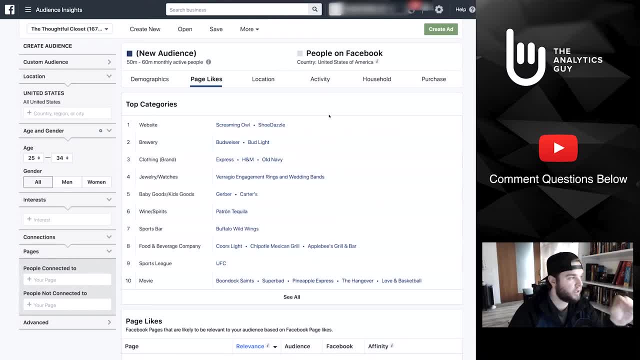 Now it's one thing that I kind of glazed over. You will need to establish, maybe an advertiser or a page that you need to get into this information. It's just like if you were going to run ads for your given channel, So, or your given platform on Facebook or what have you, but then you get access to. 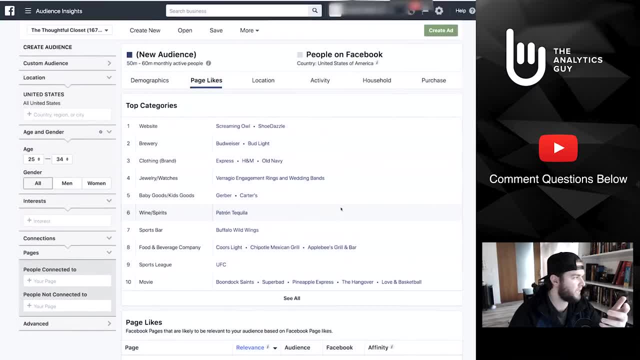 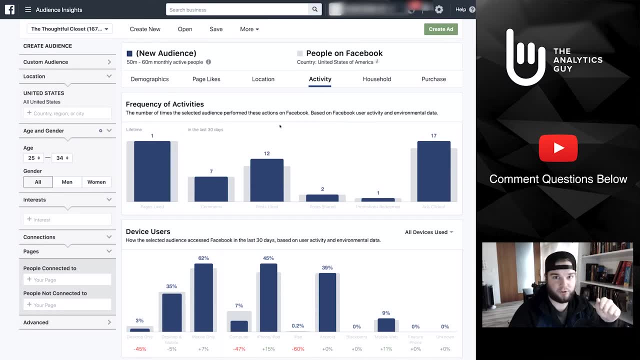 this information- There's just so much here- What pages they like on Facebook. I particularly like the activity here. So how engaged are these people? So if you want to understand a little bit of Worth It or something like that, you can start to understand here. how are they engaging? on what devices are they engaging? 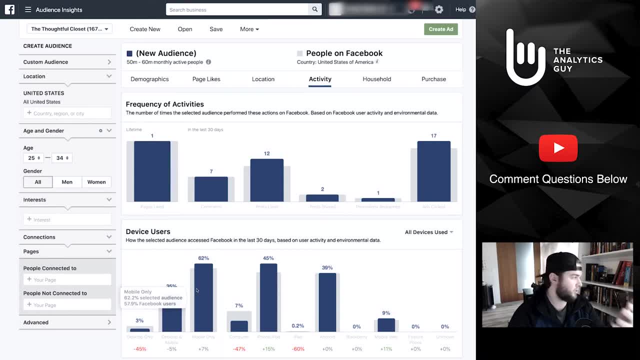 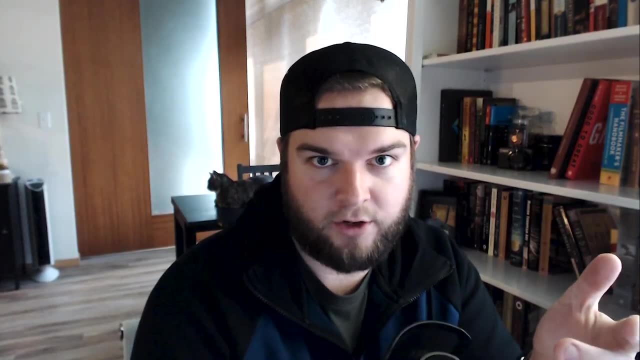 So 62% of this audience that I'm looking at- So 25 to 34 in the US- are mobile only. So let's just talk about that insight just for a second. Today's going to be a long video, guys. I'm sorry, but if you're producing content on mobile only, okay, that will have to do. 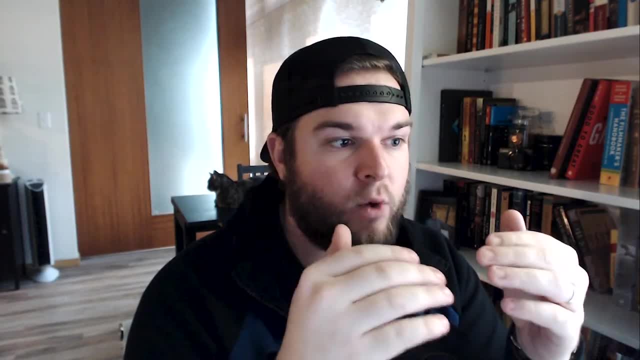 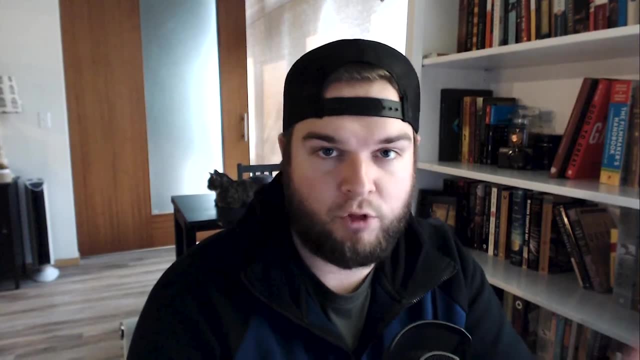 with screen size and resolutions. If you want to ask them to interact with certain things, or descriptions or cards or different things like that, you can prompt them for the platform in which you are predominantly speaking to them on right now. I would caution you to look at all the other. 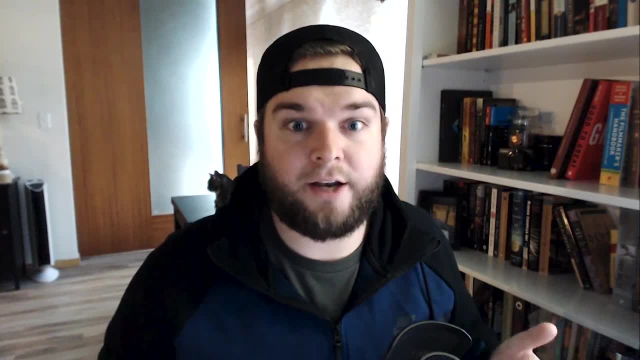 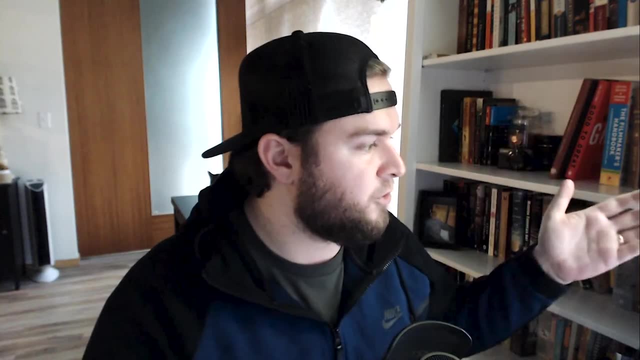 People that also make up the different parts of that audience on your platform of choice. But, for instance, if you're an Instagrammer, you might want to filter this exclusively for mobile. Why? Because, about this, many people look at Instagram on desktop. 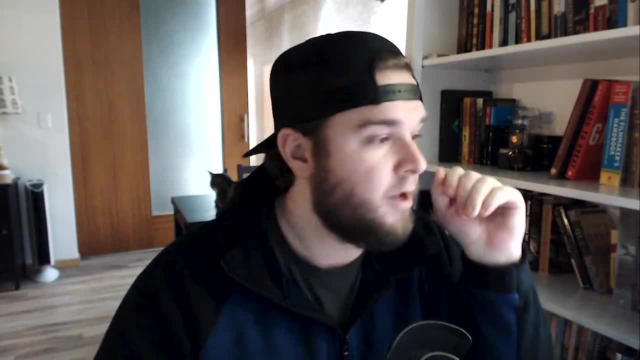 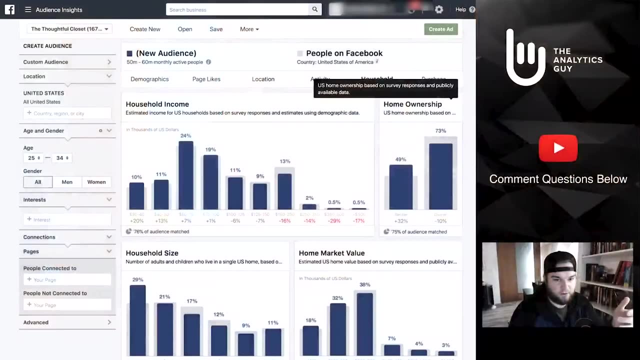 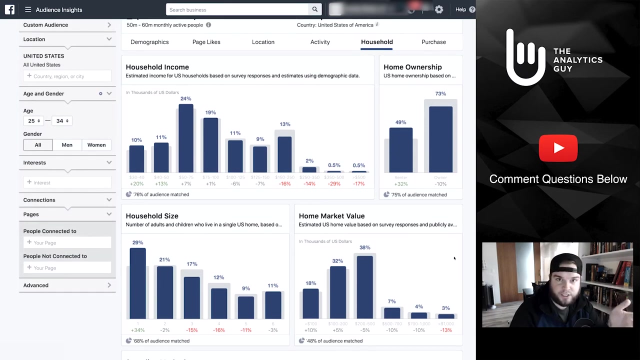 Yes, Instagram does have a desktop version, just in case you're wondering, but no one uses it. So that is a good example. or this household data. Let me flip that screen back over. Here are their medium household- Excuse me, household incomes, where you can look at the household size or different things. 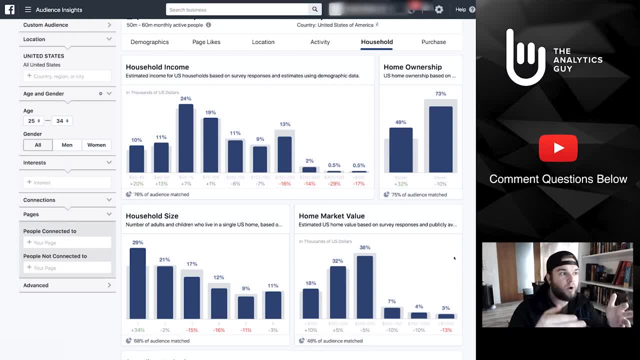 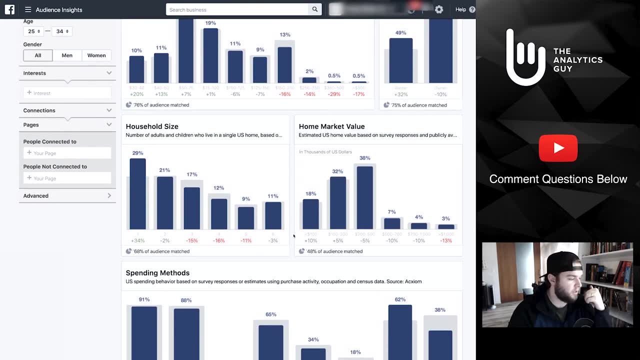 like. it is completely up to you how you want to use this information. I'm just providing you access or info about this. You know it truly exists, So how you want to creatively use this is completely up to you. There's so much information in here and there's even purchase data in here, which is great. 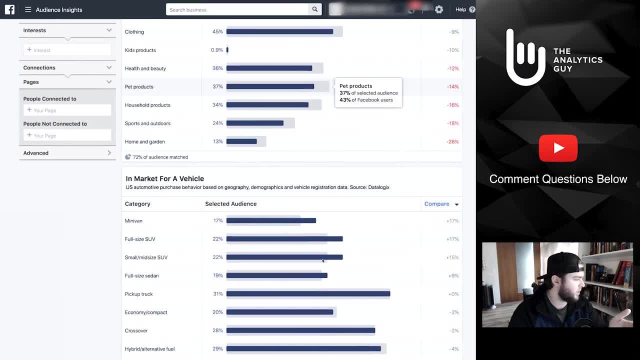 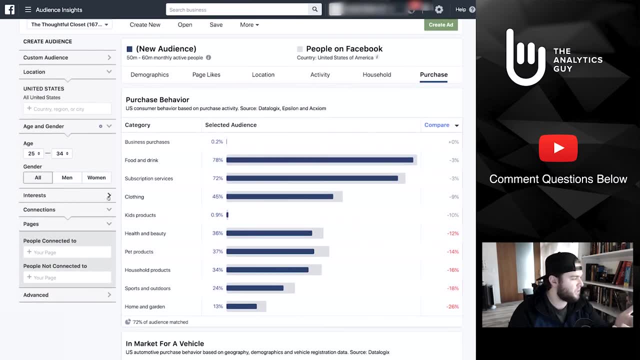 in terms of what they're purchasing, The, The list numbers associated with that, What types of vehicles do they have? There's all kinds of information in here, But the great thing is is you can always customize interests. So let's say, I want to add an interest called YouTube. 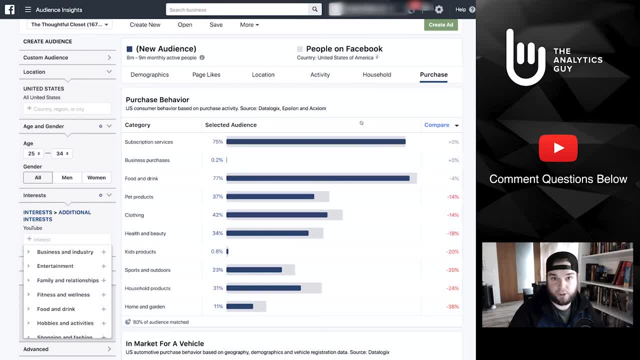 So that's something that we can sense in the data. You can see it all changes again. So maybe that's I'm looking from a YouTube perspective. They're interested in YouTube. This is using behavioral data, So it's not just someone like to YouTube on Facebook and that insinuates that they are. 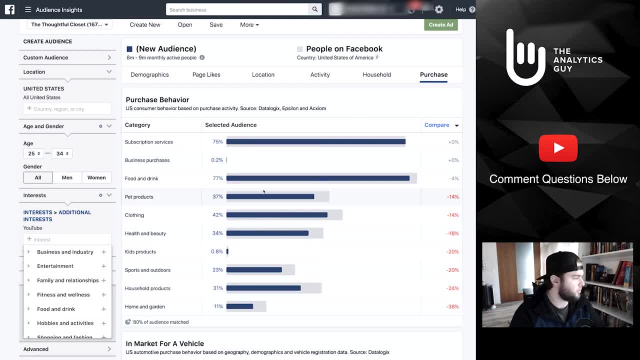 interested in YouTube. No, this very much so is using the behavioral data. When you look in here, there's all kinds of interests that you can come in here: Connections- Maybe you want to see a certain page that yours. you can see a couple here for us. 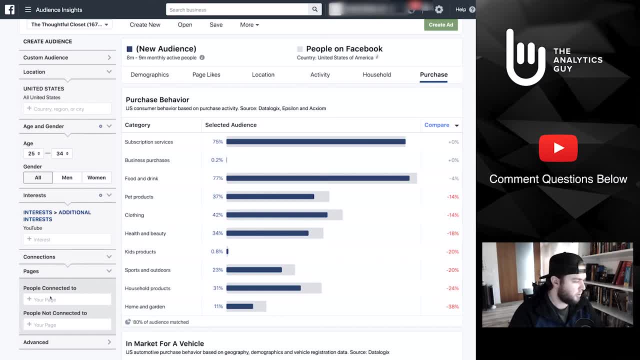 But you know there's all kinds of different filters you could put in. you know who is a negative target, So you want to understand people, that you don't want to look at the data of the people who are already following Something. there's all kinds of information in here. 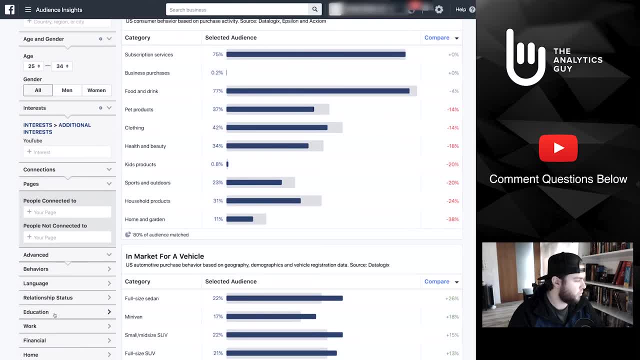 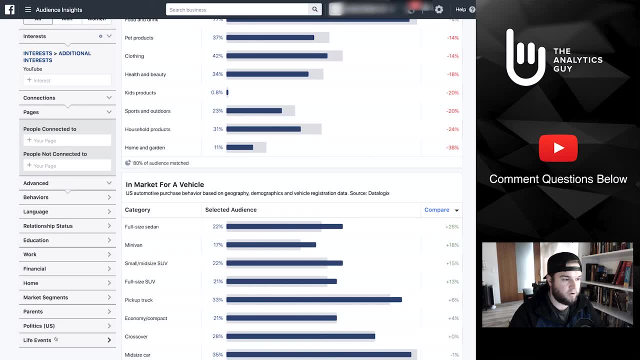 It's really great. The advanced area: These are more behaviors, relationship statuses, financials, market segments, life events. So let's say, people that are, you know, having children and you're a family vlogger, you're about to get into that world and you want to understand how to put your, you know, upcoming 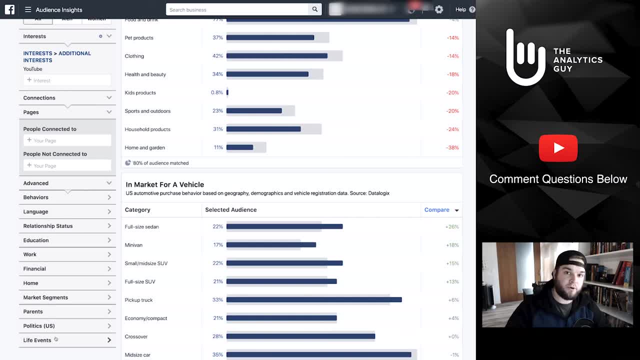 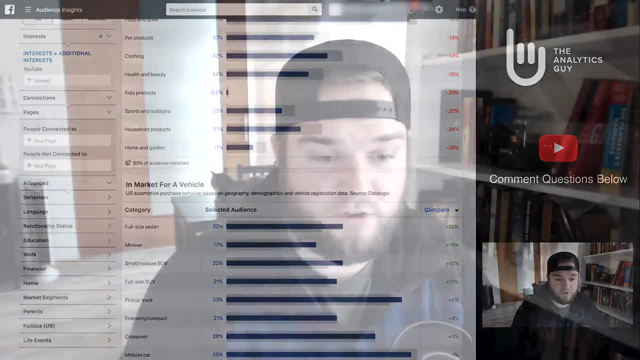 birth videos or whatever you're doing in front of the right people. This is the information that you want to use. So I've already been talking to you guys. I've been talking to you guys for like 12 minutes. There's so much information here.